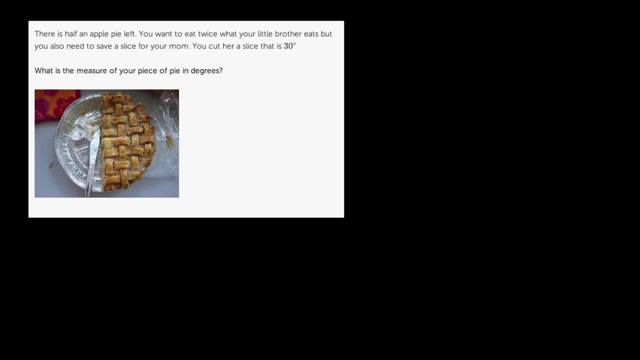 So to tackle this, we just have to remember a few things. We have to remember that the degrees in a circle. so if we were to go all the way around a circle, that that would be 360 degrees, But we only have half a pie here. 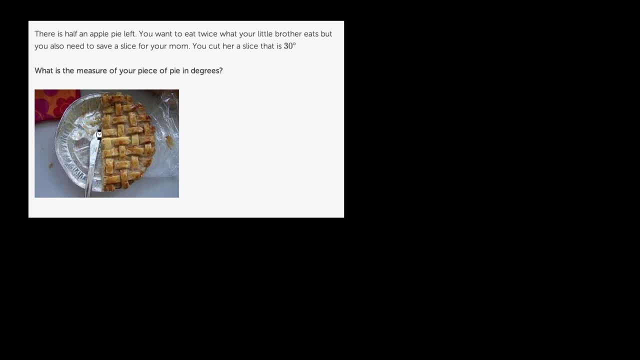 And actually let me draw it a little bit differently. So if we had a whole pie, so if we started here, if we had a whole pie, we went all the way around. that would be 360 degrees. but we only have a half pie. 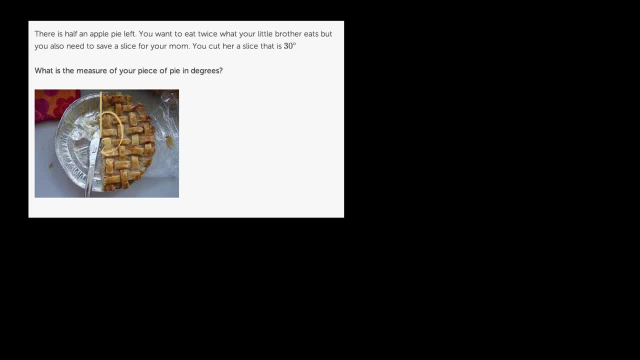 So we only have 180 degrees, And let me do that in a color you're more likely to see. That's hard to see as well. We only have 180 degrees of pie left, But let's just keep that in mind and think. 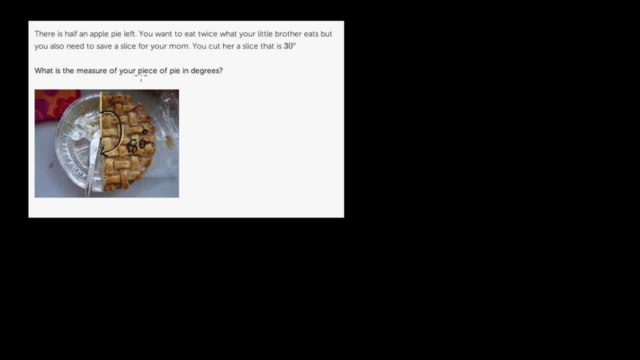 about how we're going to split it between ourselves, our brother and our mom. So let's define some variables. Let's let x be equal to the degree measure of my brother's pie or your little brother's pie. So this is degree measure of brother's pie. 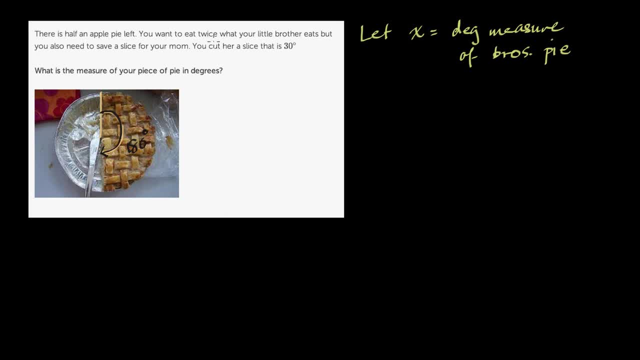 And then what would the amount of pie you eat be? Well, it says you eat twice what your little brother eats, So 2x would be equal what you eat, And it's really the degree measure of what you eat. And then, how much does your mom eat? 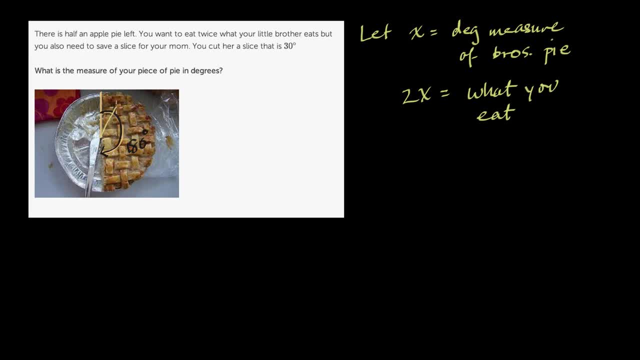 Well, it says you cut her slice that is 30 degrees. So your mom's going to get a 30-degree slice, going to get a slice, something like that. So the amount that your brother eats, x plus the amount you eat, plus the amount that your mom gets, plus 30 degrees. 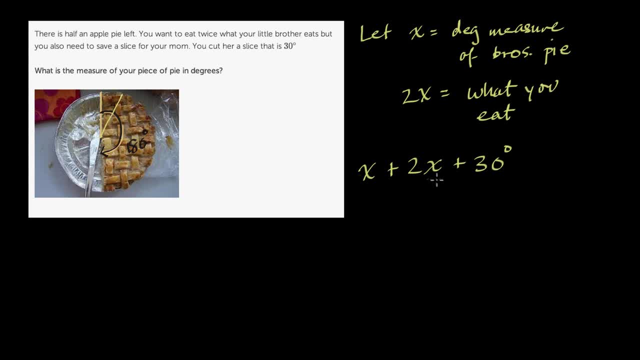 is going to be equal to this, This half pie, And remember, all of these are degree measures, So it's going to be equal to 180 degrees. And just to visualize it over here, and let me do it down here where it's easier to see it- 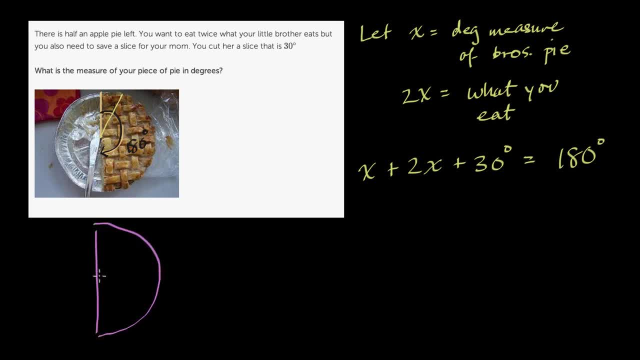 We have half a pie that we're dealing with. We're going to save 30 degrees for our mom, So that's 30 degrees. right over there, Your brother is going to eat some amount, So that is x, And then you're going to eat twice. 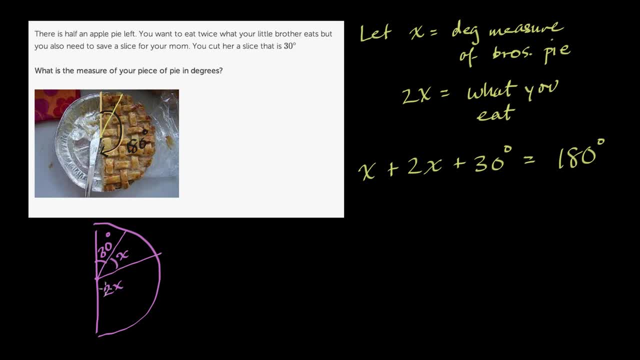 that amount. so that is 2x. x is the measure of this angle And then 2x is the measure of that angle. So you see that 30 degrees plus x plus 2x, or x plus 2x plus 30 degrees is going. 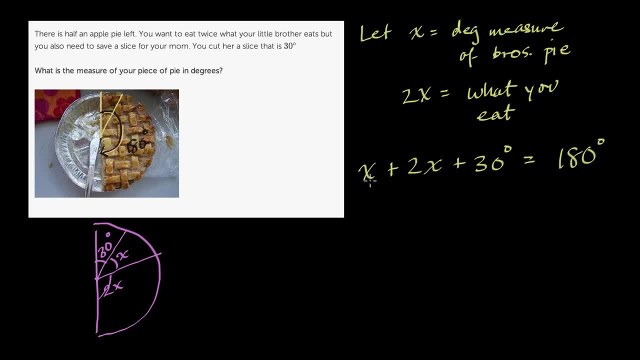 to be equal to 180 degrees. Now we can simplify this. If we have one of something and then have another two of it, how much do we have now? Well, I now have 3x's, So 1x plus 2x's is going to be 3x's. 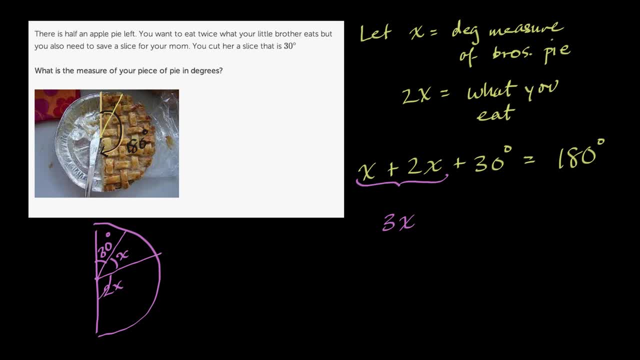 So I have 3x plus 30 degrees. Plus 30 degrees is going to be equal to, of course, 180 degrees. Now to solve for x, we can subtract 30 degrees from both sides. So minus 30 degrees, minus 30 degrees. 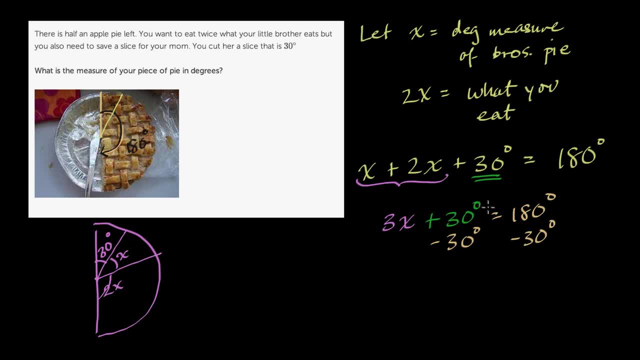 And I could have just written the. I could have all assumed that I'm doing it in degrees and just done it at the end. But I keep writing it, so I'll just keep going with that. And then we are left with 3x. 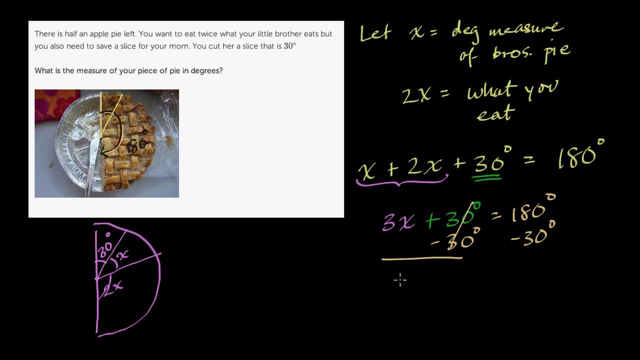 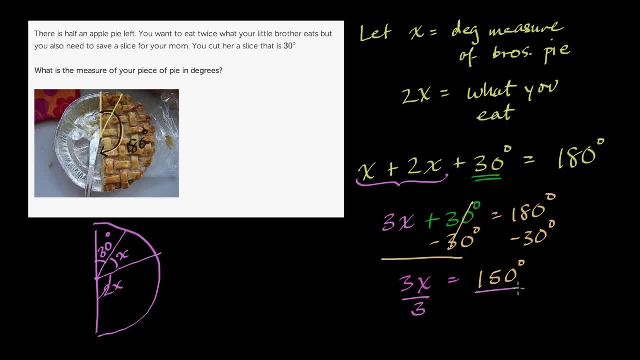 And now we can just divide both sides by 3.. And we're left with x equaling 150 divided by 3 is 50 degrees. x is equal to 50 degrees. Now we have to be careful. x is not what they're asking for. 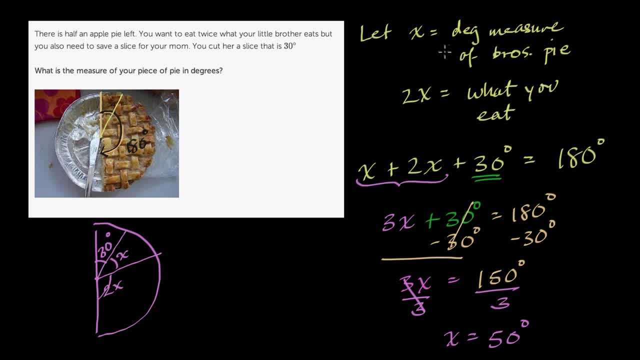 They're asking for the measure of your piece of pi in degrees. x is the degree measure of your brother's piece of pi. What you eat is 2 times that. So if x is 50 degrees 2 times, that is going to be 100 degrees. 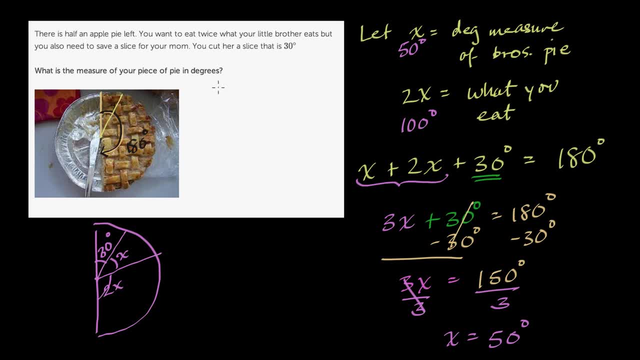 So what is the measure of your piece of the pi in degrees? It is going to be 100 degrees. So if we draw our pi again, if we draw our half pi, you have 30 degrees for your mom. So that's 30 degrees for your mom. 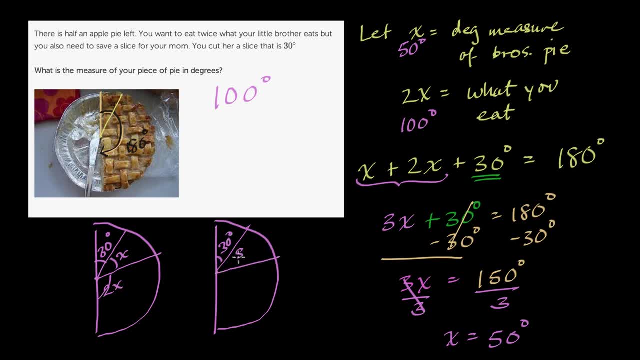 You have 50 degrees for your brother, You have 50 degrees for your brother, And then you have twice that for yourself: 100 degrees.